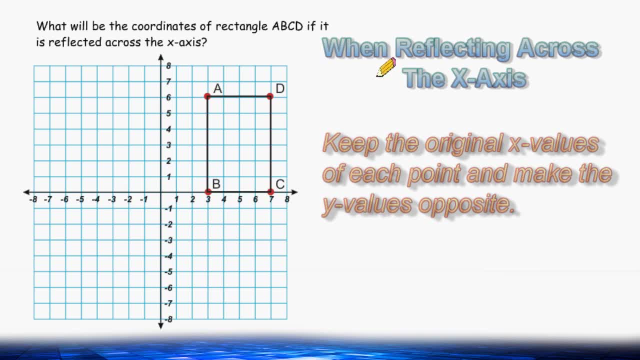 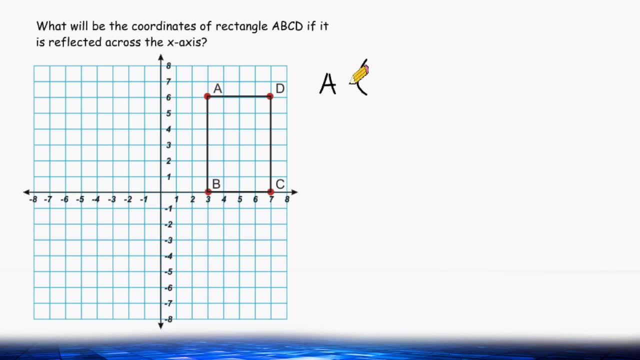 become opposite of what they are. So the first thing that we're going to do is just record the original points. And point A is located at positive 3, positive 6.. Point B is located at positive 3, 0.. Point C is located at positive 7, 0.. And point D is located at positive 7,. 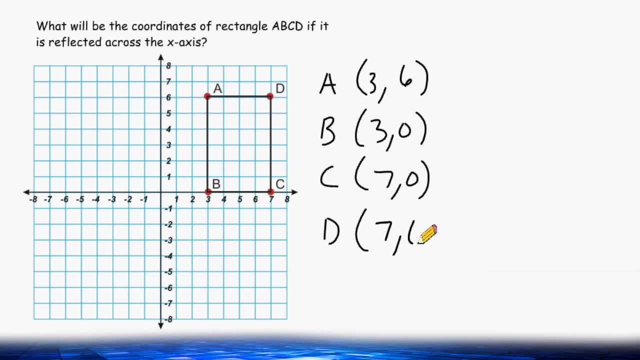 positive 6.. Now the next thing that we want to do is keep all of the X values the same. So for point A, this 3 is going to be the same and make all of the Y values opposite. So the opposite of positive 6 is negative 6.. So for B, the transformed point is going to be 3 and the 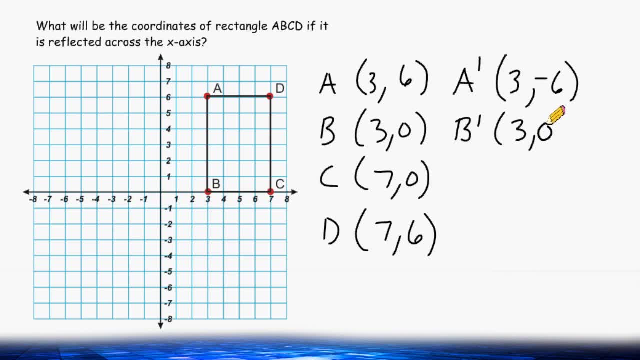 opposite of 0 is actually itself a 0. And for C, the point is going to be 7 and 0. And for D, the new location will be positive 7 and negative 6. Now that we have our new coordinates, let's plot them on the coordinate plane. So we have. 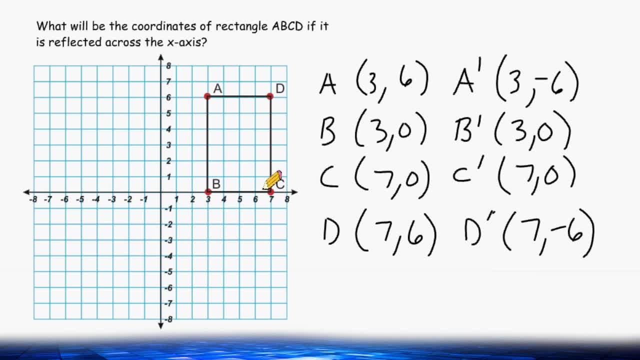 to plot the new point: A at 3, negative 6. And let's make sure to label this A. And for B: B is located at 3, 0.. Notice that it did not move from its original spot because it is. 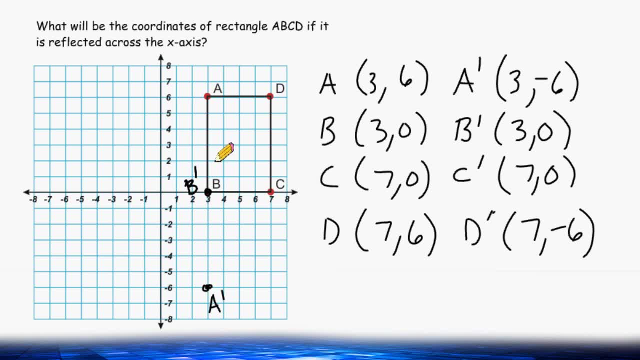 right on the x-axis And for C that is going to be right here. Eate point D is right here And point C is located at 3, 0. And for D it is located at 3.. B is located at 3, 0. And for H it's located right on the x-axis. So that really means. that point is right on the x-axis. That point did not move as well because it is also on the x-axis and point D is 7, negative 6, which is right here. And the next thing to notice about this point is that it is not moving from the y-axis all. 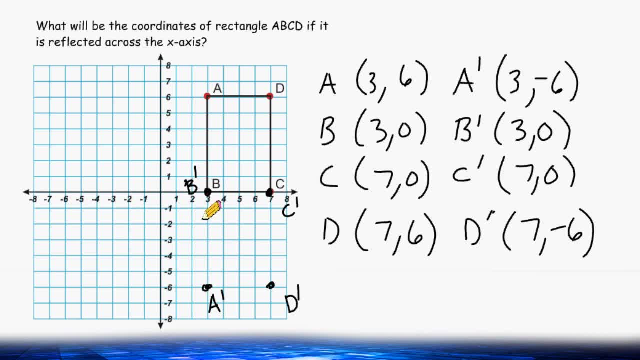 but on the positive Falckveil case, This points of all of the values are notatrexialactive. that we have to do is connect our points together to form our shape, And this is the reflected rectangle across the x-axis And these are the coordinates right here that represent the